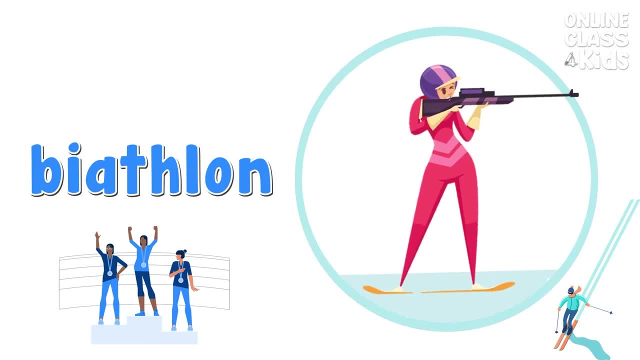 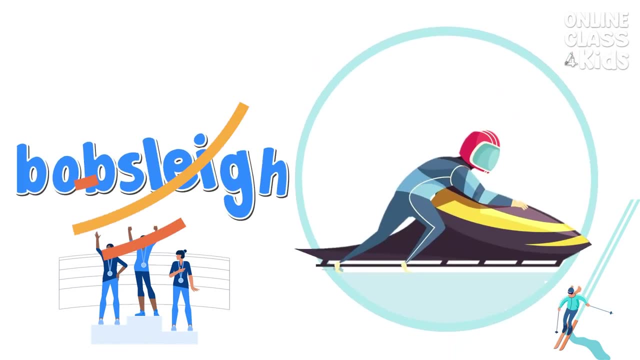 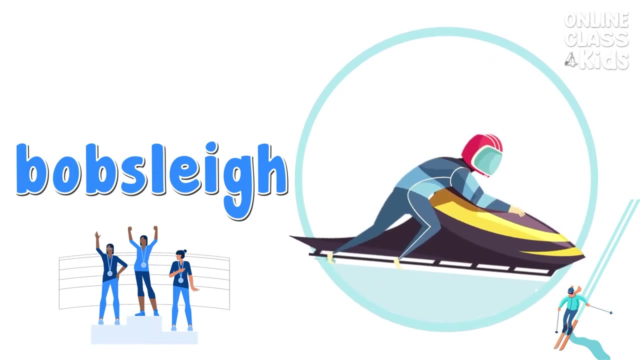 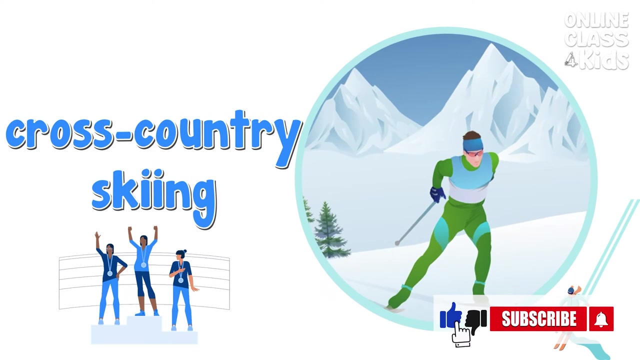 Biathlon, A sport combining cross-country skiing and sharpshooting. Say Biathlon. Bobsleigh, A sport where the fastest bobsleigh to cross the finish line is the winner. Say Bobsleigh. Cross-country skiing, A sport of skiing over fields or through woods, Say Cross-country skiing. 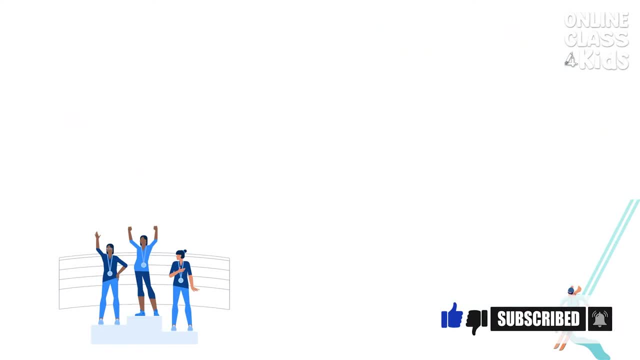 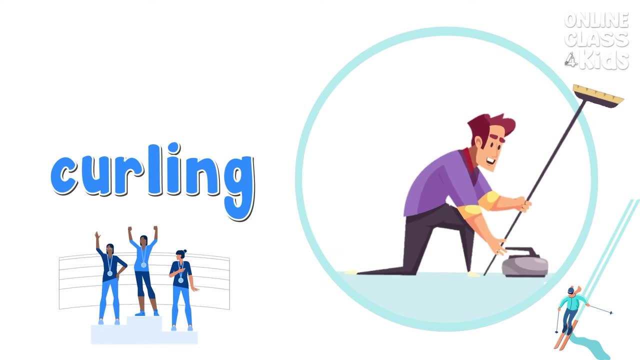 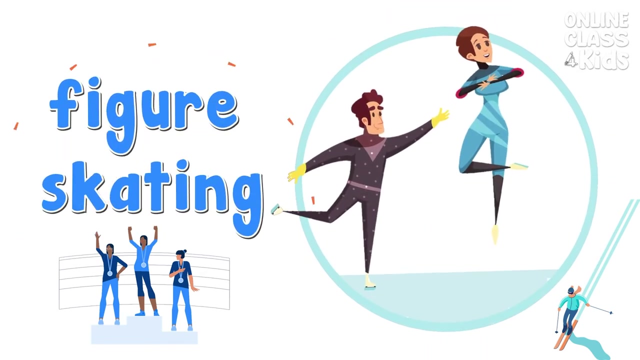 Say Cross-country skiing, A sport of skiing over fields or through woods, Say Cross-country skiing, Cross-country skiing. Curling, A team sport where they slide stones towards a target of four circles. Say Curling. Figure Skating, A sport where ice skater skates by the performance of jumps, spin and dancing: Say Figure Skating. 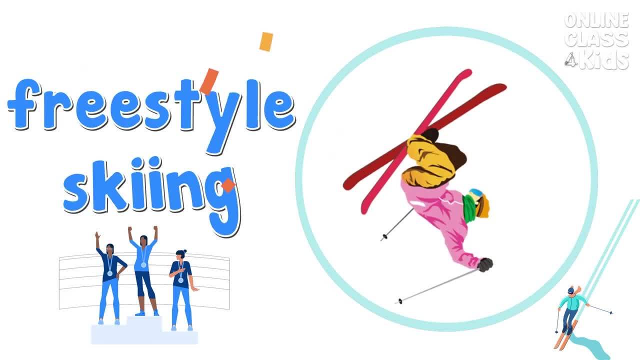 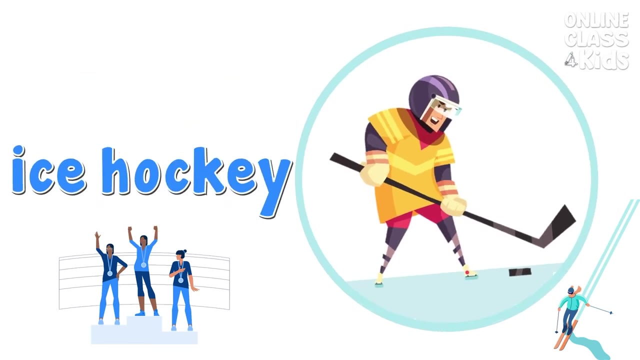 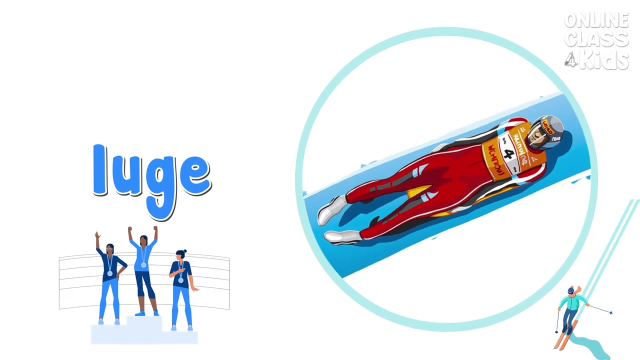 Freestyle Skiing, A sport that combines skiing and on-air tricks. Say Freestyle Skiing. Ice Hockey, A sport played using a long stick hitting a flat disc to goal. Say Ice Hockey. Loose, A sport which is led to race on a prepared downhill run for the fastest. 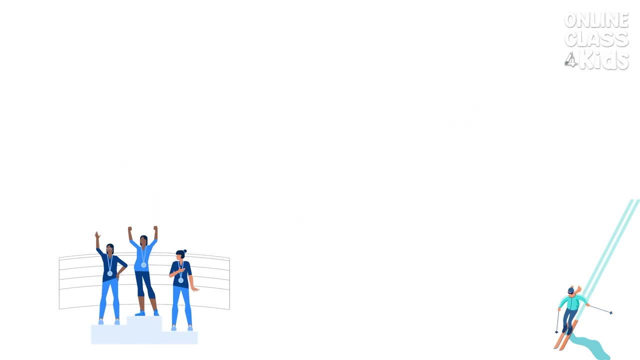 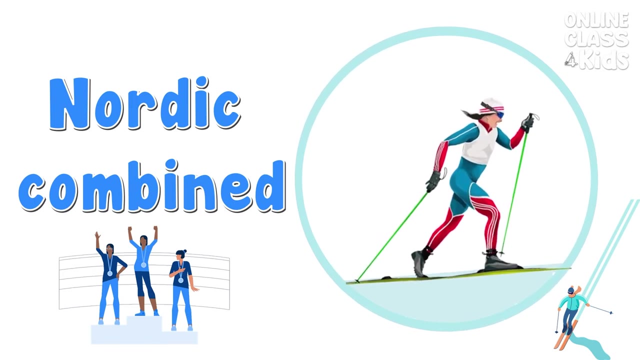 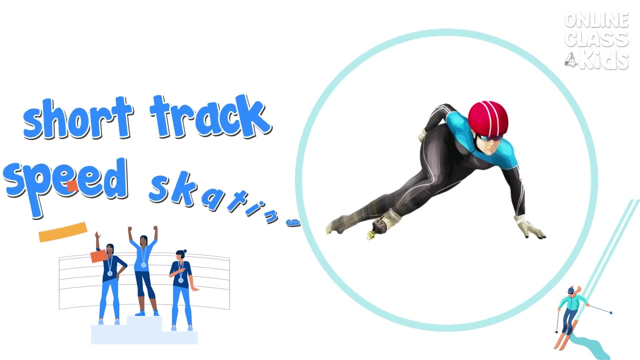 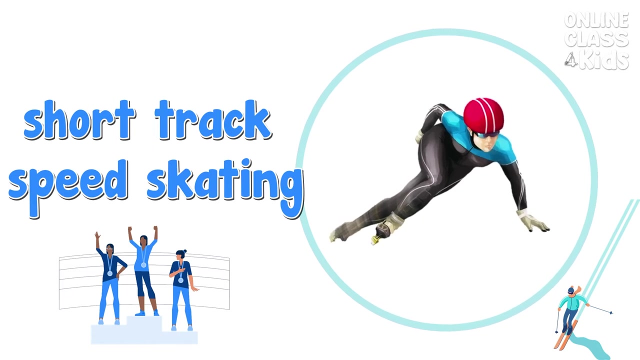 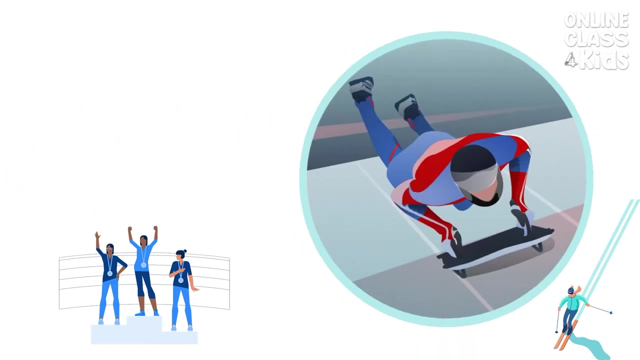 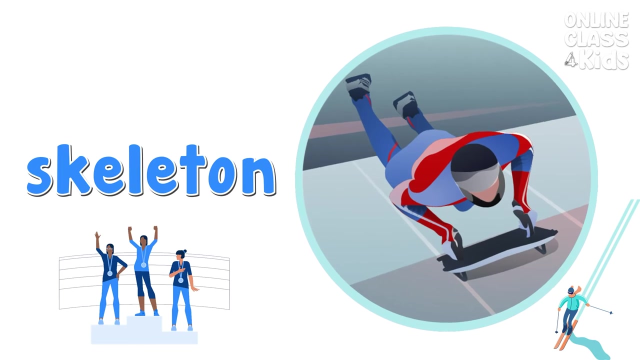 Say Loose Nordic Combined, A ski sport of both ski jumping and cross-country racing. Say Nordic Combined- Short Track Speed Skating, A sport for ice speed skaters racing Who'll cross the first line. Say Short Track Speed Skating- Skeleton, A sport using a small sled called Skeleton, while lying face down. 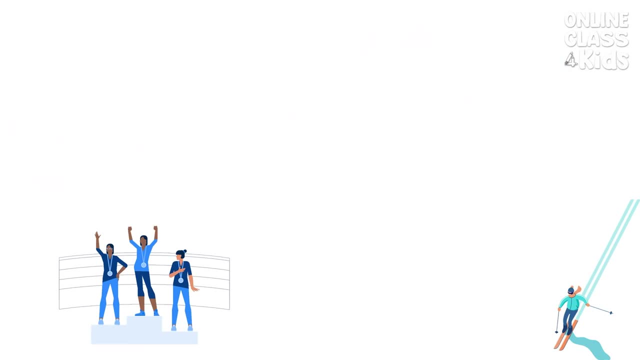 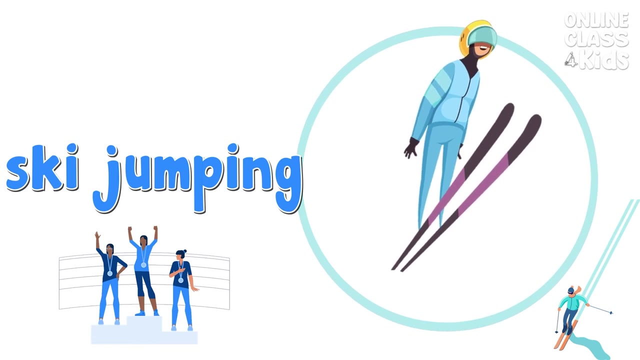 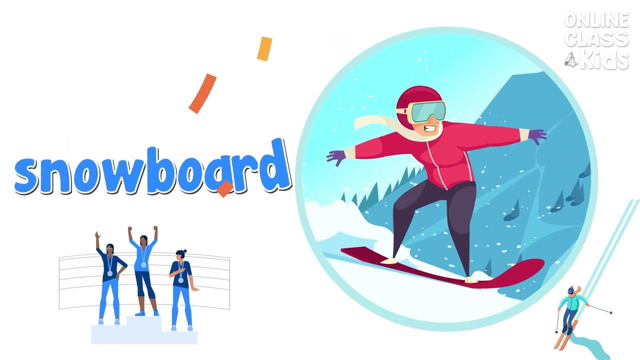 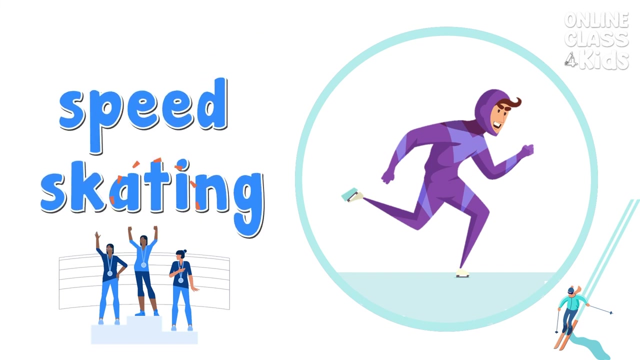 Say Skeleton Ski Jumping, A sport where skiers show their jump styles reaching farthest. Say Ski Jumping Snowboard, A sport using a large skateboard that one can ride it down a hill over snow. Say Snowboard Speed Skating, A competitive ice skating sport which skaters wear speed skates and race.